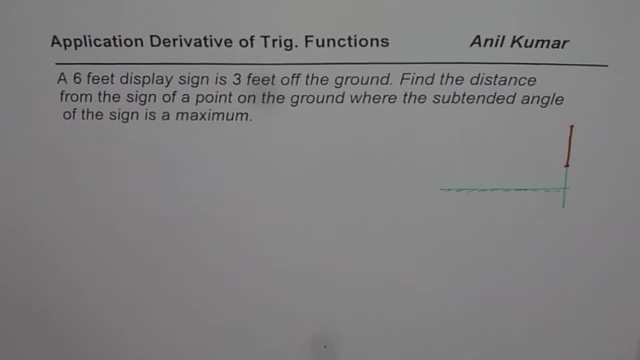 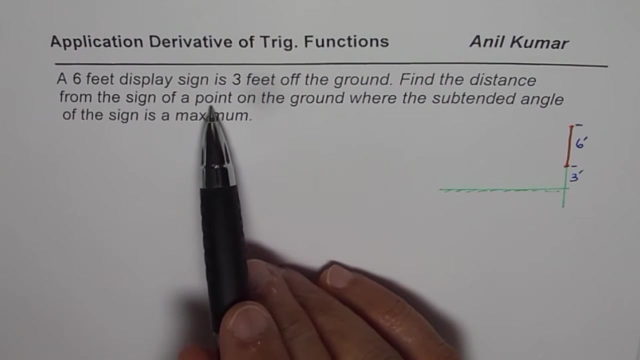 And what is given to us is that this display sign is 3 feet off the ground, So it is 3 feet off the ground, And 6 feet is the display sign itself, So that is 6 feet. Find the distance from the sign of a point on the ground where the substantive angle of the sign is maximum. 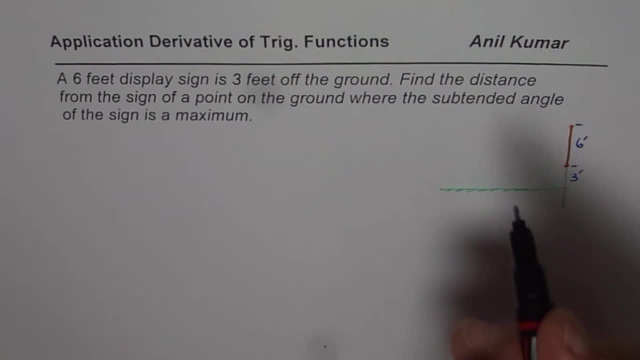 So what we need to find is a point on the ground, So we need to find the distance from the sign of a point on the ground, Somewhere on this ground where the angle which this picture makes is maximum, Kind of like this: 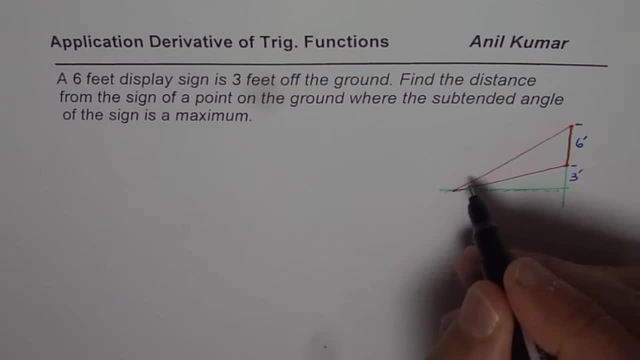 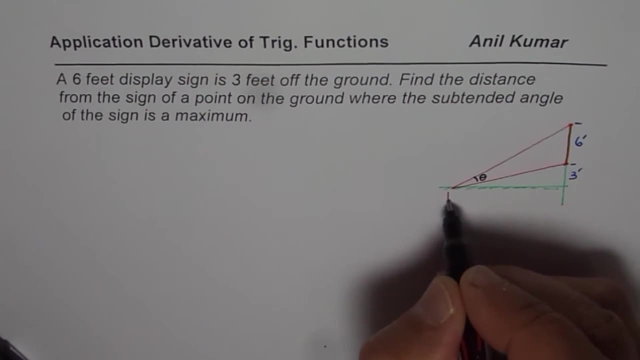 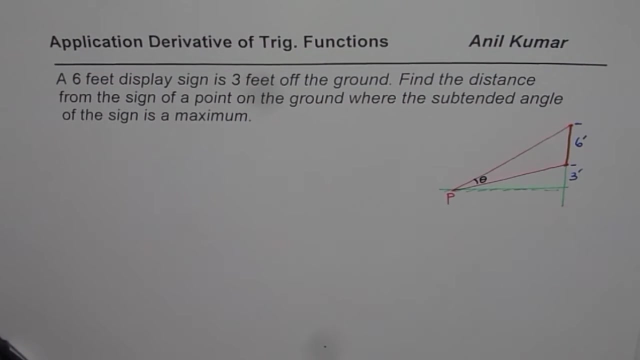 So we are looking for the angle, theta, let us say, to be maximum, So some point on the ground, let us call this point as p, right? So that is the question for us. We need to maximize the sight, this angle, right? 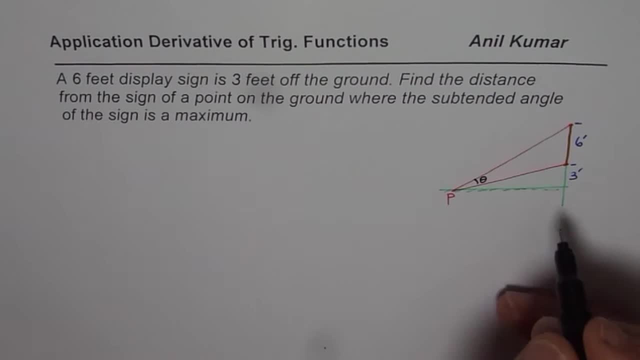 So that is the question. I hope it is absolutely clear. Now let me write down, label this a bit: A, B and let us say C, right? So that is the picture A to B, 6 feet, 3 feet above the ground. 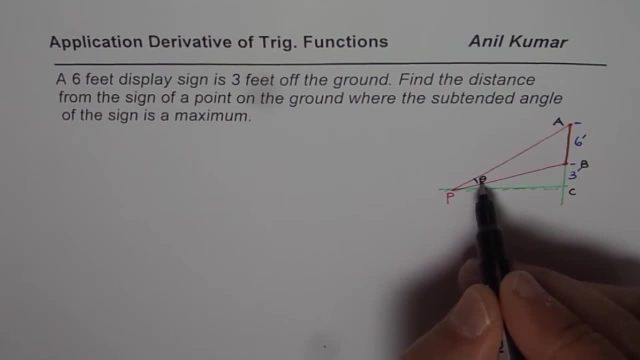 Point P is on the ground and we want to maximize the angle theta. So we want to find what is this distance X from where this point will be, from where maximum angle theta is possible. So this is the question for you. 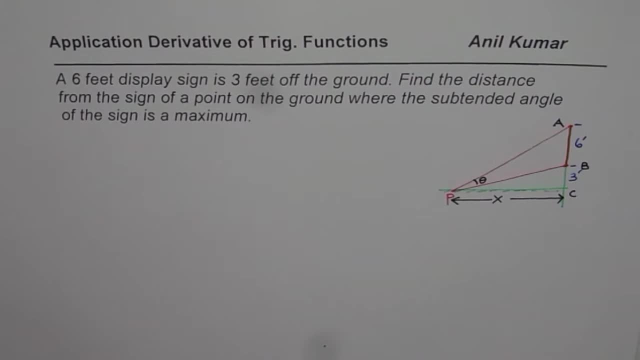 How are you going to solve it? You can still pause the video, answer the question and then look into my suggestion, right? Well, to solve this question, we will use trigonometric functions, and let us see how they make the job so simple for us. 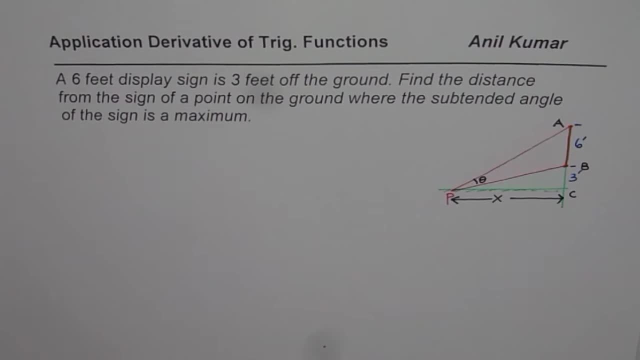 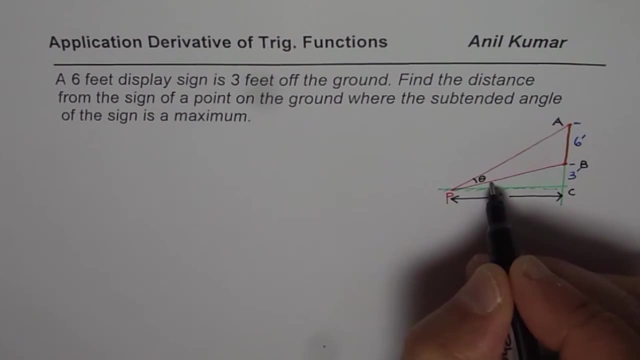 Otherwise, this is indeed a very difficult question. So what we will consider is: we want to maximize this angle. Let us say that this small angle is- let me use a different ink. let us say that this small angle is alpha right. 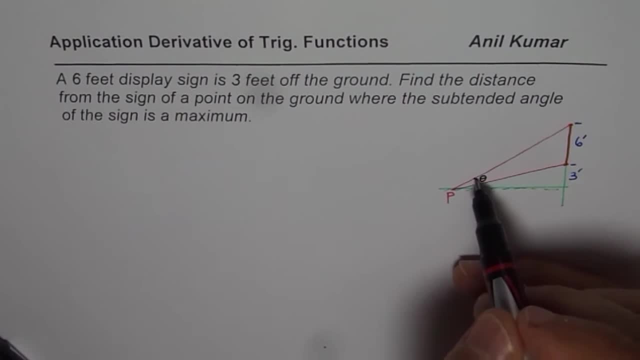 That is the question for us. We need to maximise the site, This angle. So that is the question. I hope it is absolutely clear. Now let me write down. label this a bit: A, B and let us say C. right, 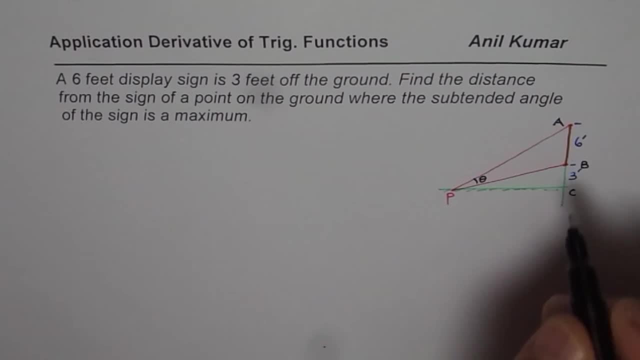 So that is the picture A to B: 6 feet, 3 feet above the ground. Point P is on the ground and we want to maximize the angle theta. So we want to find what is this distance X from where this point will be? 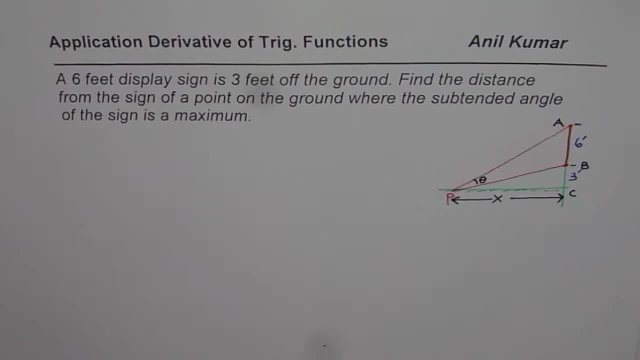 from where maximum angle theta is possible. So this is the question for you: How are you going to solve it? You can still pause the video, answer the question and then look into my suggestion right. Well, to solve this question, we will use trigonometric functions. 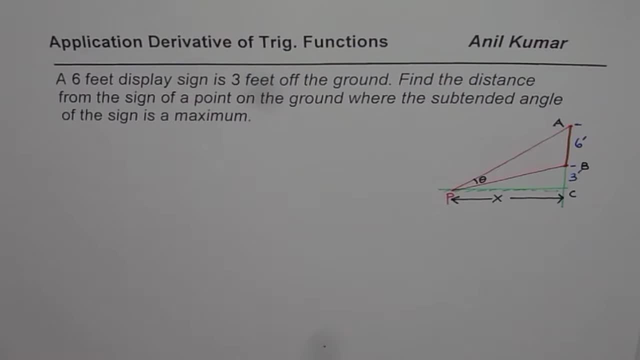 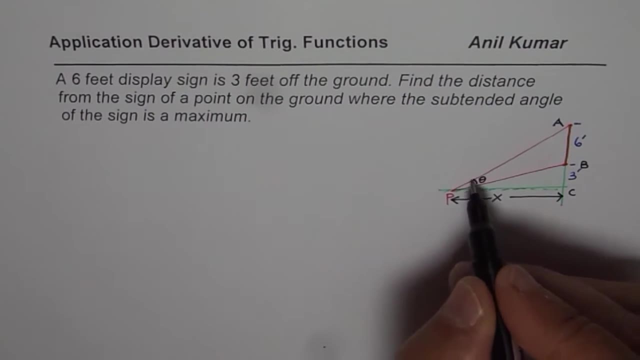 and let us see how they make the job so simple for us. Otherwise, this is indeed a very difficult question. So what we will consider is: we want to maximize this angle. Let us say that this small angle is- let me use a different ink- 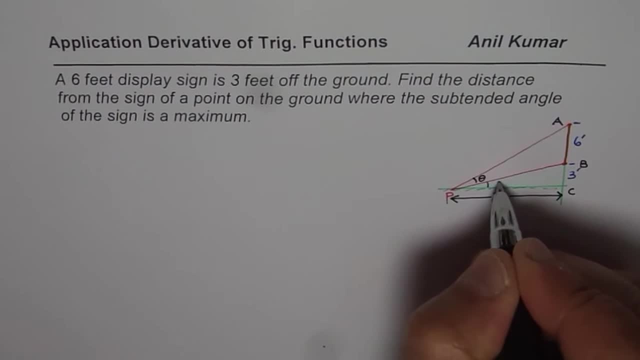 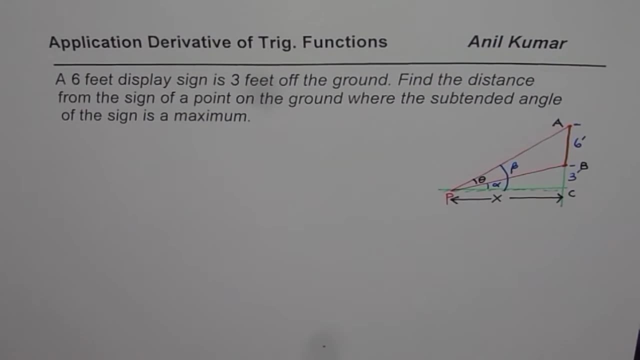 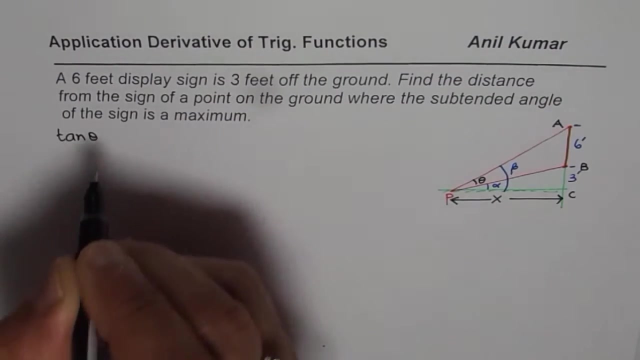 let us say that this small angle is alpha right And the big angle here is beta. okay, In that case you can write tan of theta. you can write tan of theta as equal to theta is beta minus alpha right. 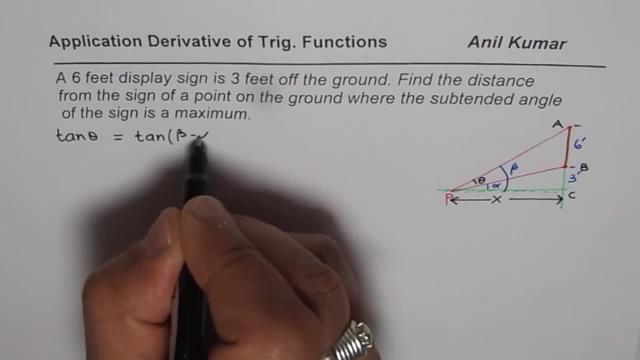 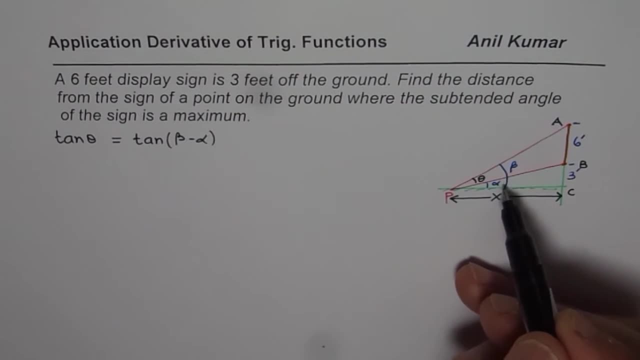 Which is equal to tan of beta minus alpha, right? I hope that point is very clear, right? So this angle, theta could be beta minus alpha. that's clear. So tan of theta is same as tan of beta minus alpha. 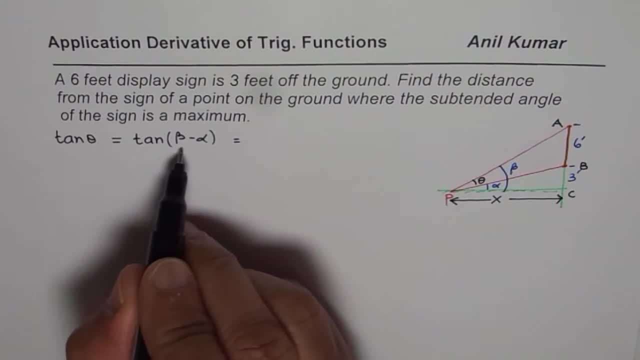 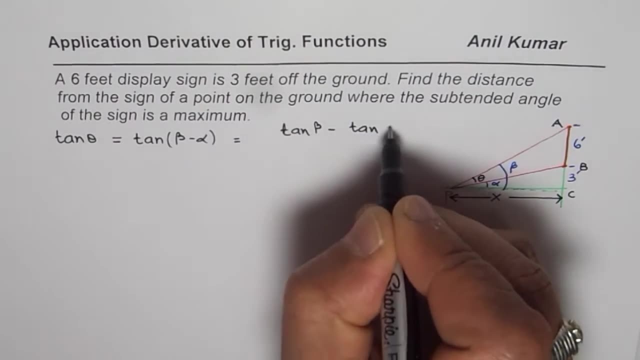 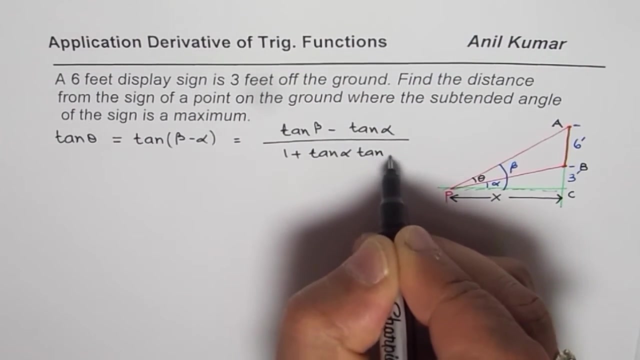 Now, if you remember the trigonometric formula, what is tan beta minus alpha? That is tan beta minus tan alpha, divided by 1 plus tan alpha, tan beta, Right, So you could have written beta or alpha, the order doesn't matter here. okay. 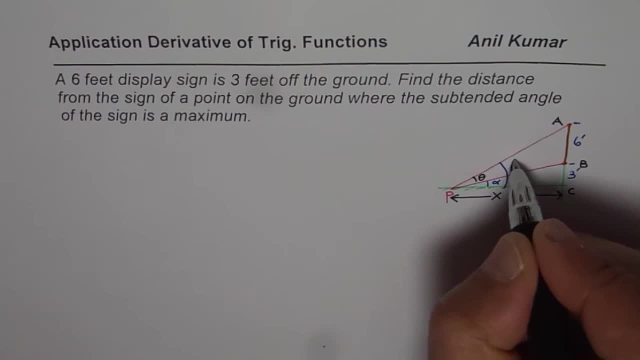 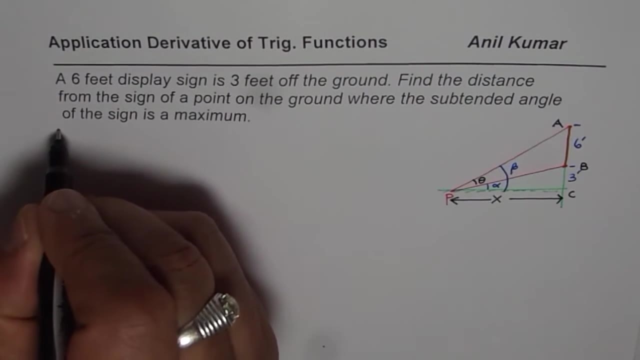 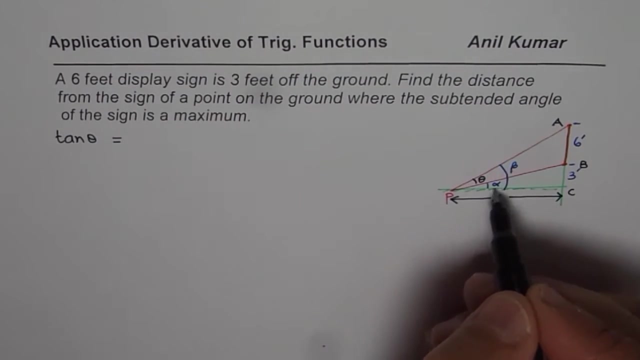 And the big angle here is beta. okay, In that case you can write tan of theta. you can write tan of theta as equal to: theta is beta minus alpha right, Which is equal to tan of beta minus alpha right. 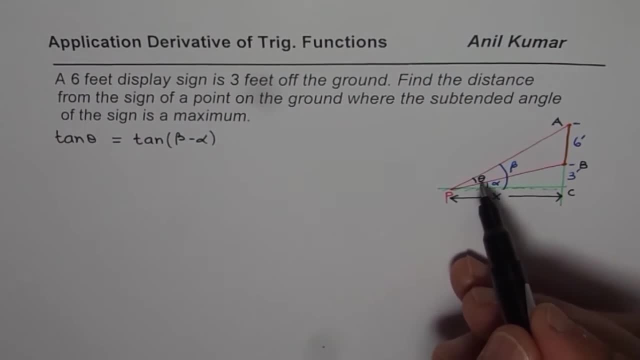 I hope that point is very clear, right? So this angle, theta could be beta minus alpha. that's clear. So tan of theta is same as tan of beta minus alpha. Now, if you remember the trigonometric formula, what is tan, beta minus alpha? 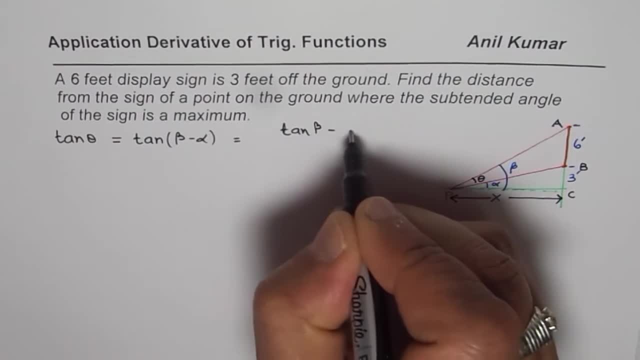 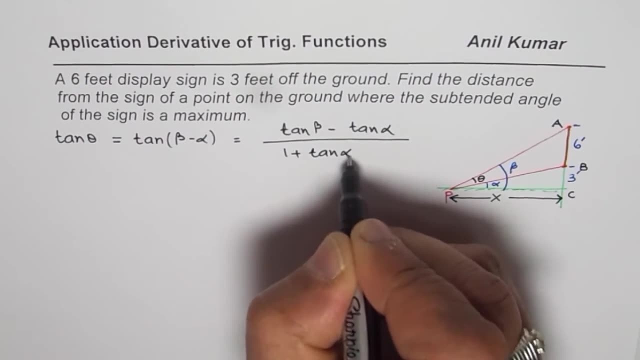 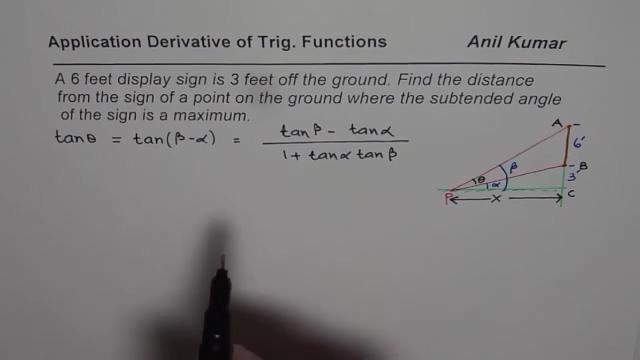 That is tan beta minus tan alpha, divided by 1 plus tan alpha, tan beta. Right, So you could have written beta or alpha, the order doesn't matter here. okay, So that is first part. Now, in this case, what is tan beta? 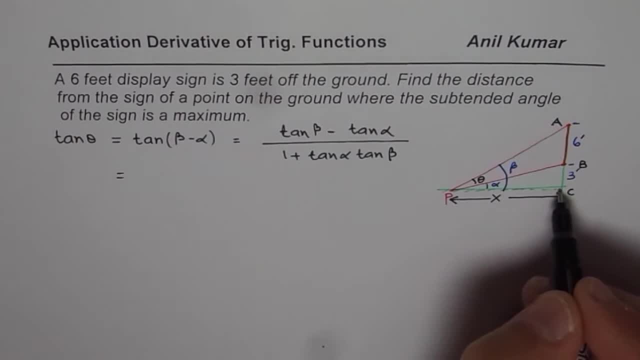 Tan beta is this big triangle, if you see, is that side AC, which is 6 plus 3,, 9, right. So this side is 9 for us. So, tan, you know, is opposite, over adjacent side. 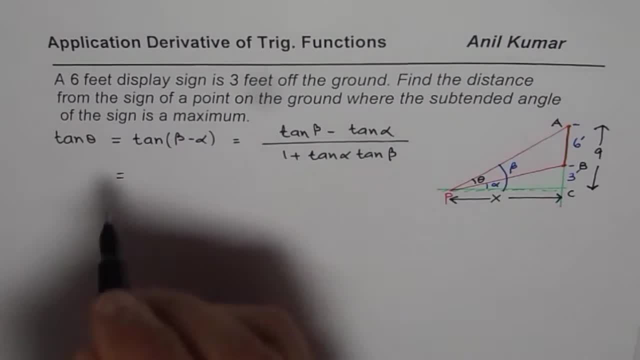 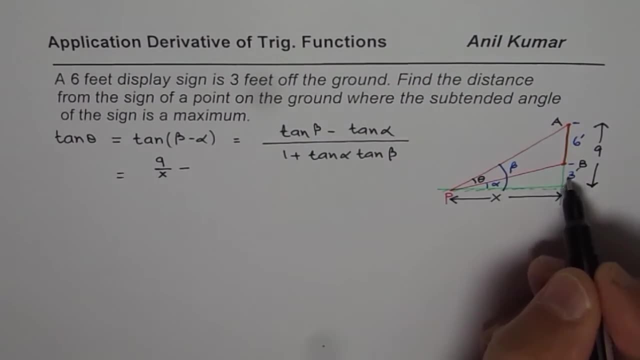 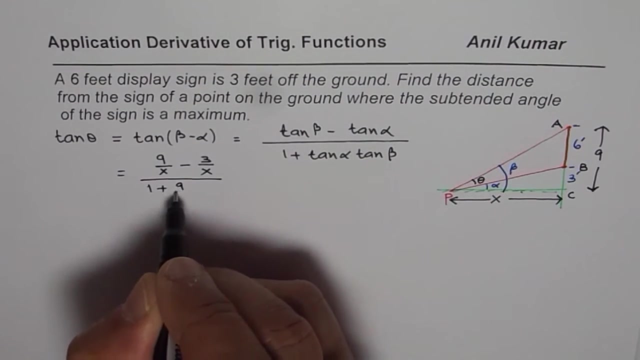 So tan beta is 9 over x. So instead of tan beta, tan beta is 9 over x. So I will write 9 over x minus tan of alpha. this small triangle is 3 over x, So 3 over x divided by 1 plus 9 over x times 3 over x. 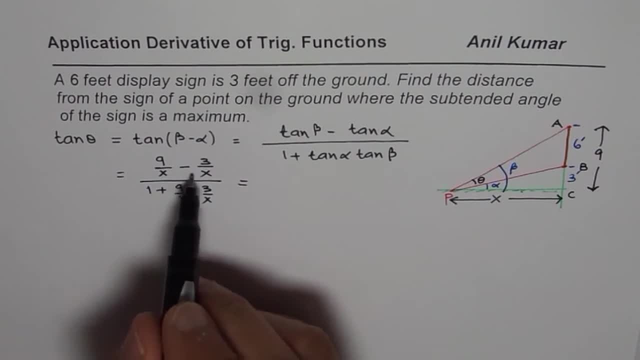 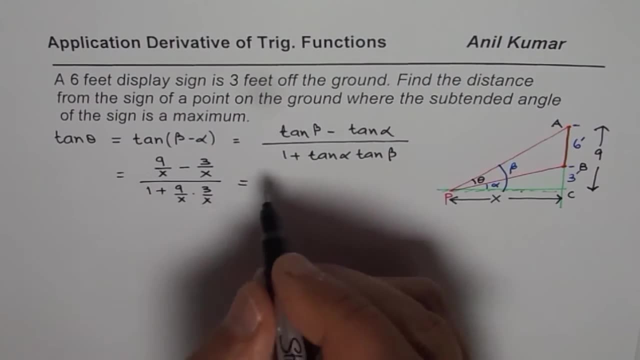 Let's try to simplify this. Common denominator is x here, So what we will do is we can just multiply by x squared, So we'll get 9x minus 3x, which is 6x, 6x in the numerator divided by. 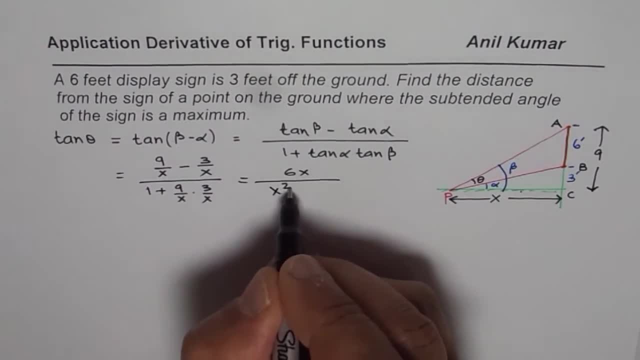 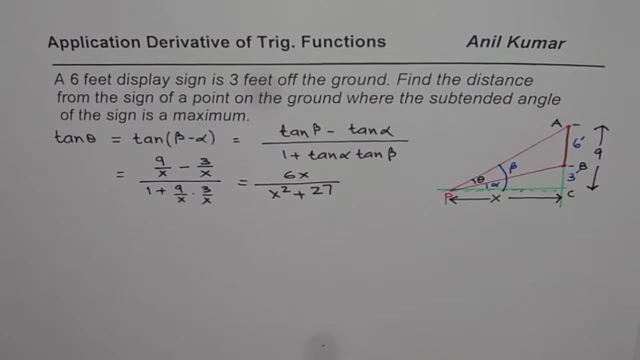 if you multiply by x squared, you get x squared here right, Plus x squared cancels 9 times 3, 27.. This is what you get. All this is equal to tan theta. Perfect. Now we have two variables to work with. 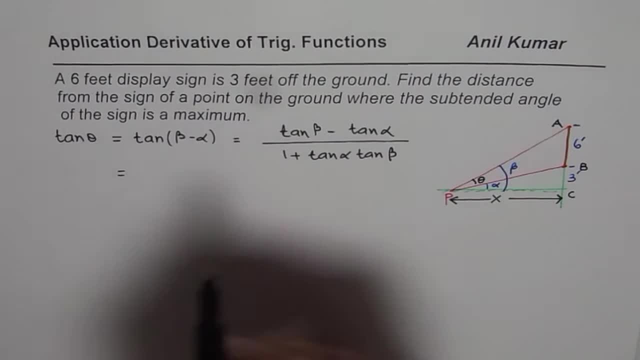 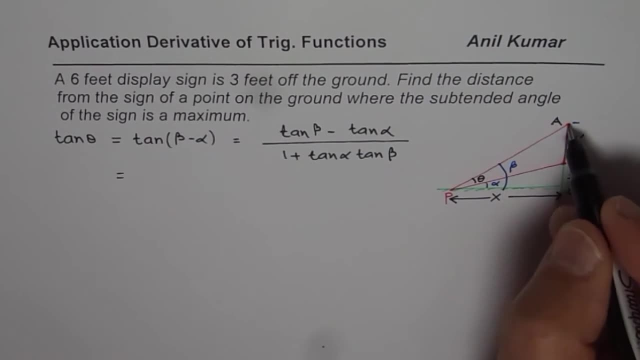 So that is first part. Now, in this case, what is tan beta? Tan beta is this big triangle, if you see, is that side AC, which is 6 plus 3,, 9, right? So this side is 9 for us. 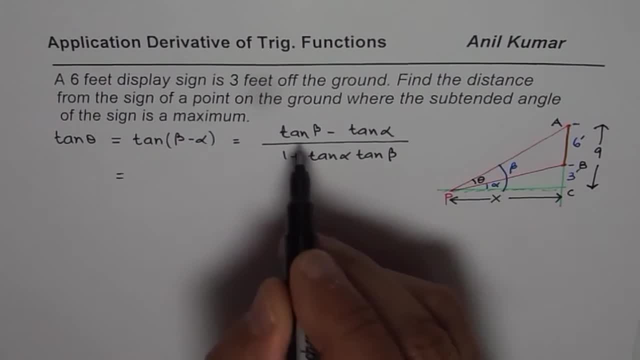 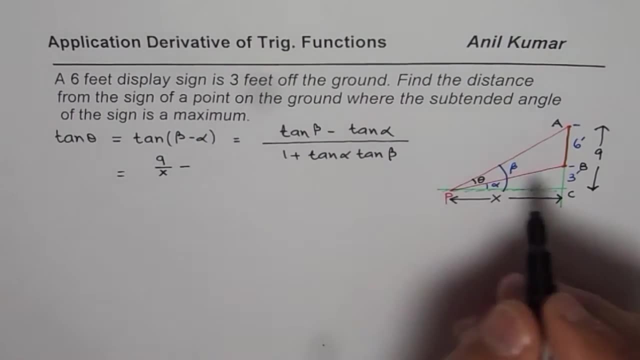 So tan, you know, is opposite over adjacent side. So tan beta is 9 over x. So instead of tan beta, tan beta is 9 over x. So I will write 9 over x. minus tan of alpha, this small triangle is 3 over x. 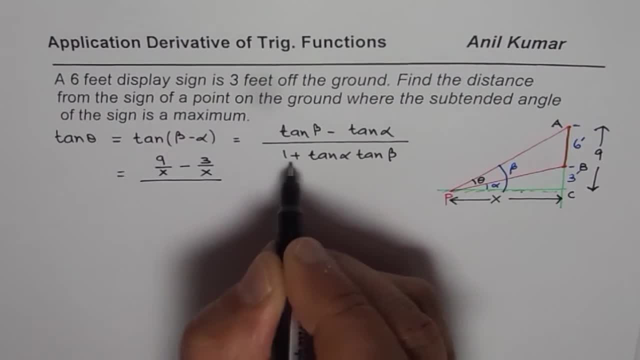 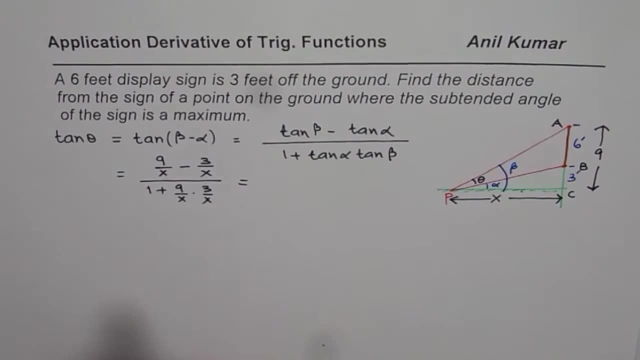 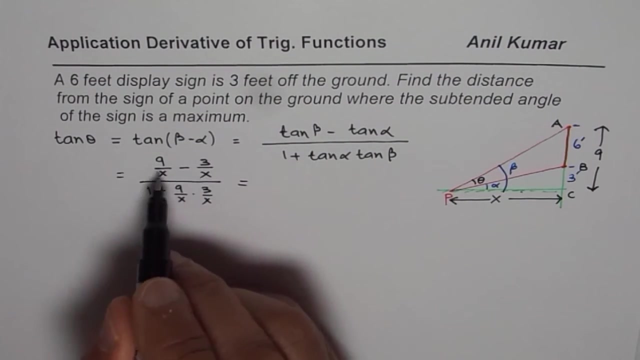 So 3 over x divided by 1, plus 9 over x times 3 over x. Let's try to simplify this. Common denominator is x here, So what we will do is we can just multiply by x squared, So we'll get 9x minus 3x, which is 6x. 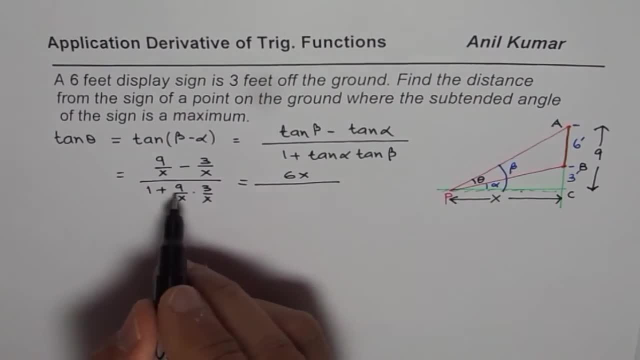 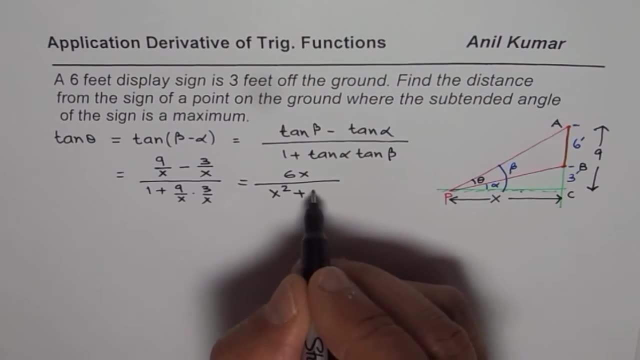 6x in the numerator divided by. if you multiply by x squared, you get x squared here, right. Plus x squared cancels 9 times 3, 27.. This is what you get. All this is equal to tan theta. 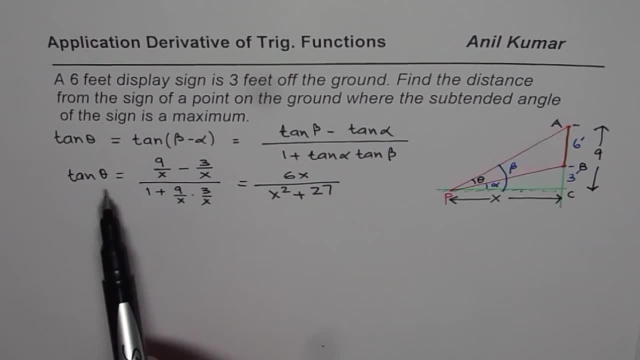 Perfect. Now we have two variables to work with: theta and the angle x. We can take derivative with respect to x. that is our function, right? So we can take derivative with respect to x on both sides. So at this stage we are taking derivative. 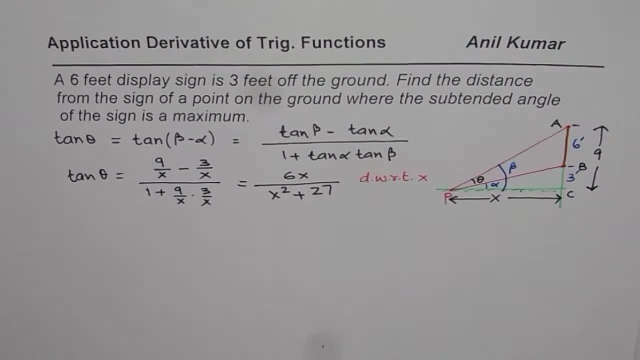 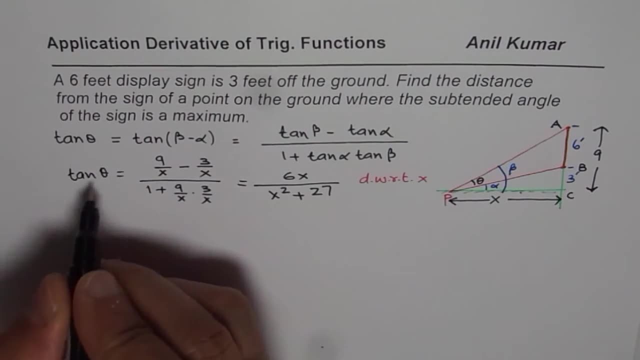 with respect to x right on both the sides. So in that case, what do you get? So you get derivative of tan theta secant squared theta. So we get secant squared theta times d theta. dx right Equals 2.. 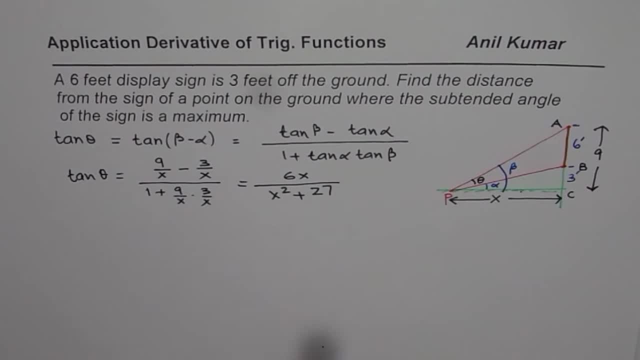 theta and the angle x. We can take derivative with respect to x. that is our function, right. So we can take derivative with respect to x, with respect to x, on both sides. So at this stage we are taking derivative with respect to x. 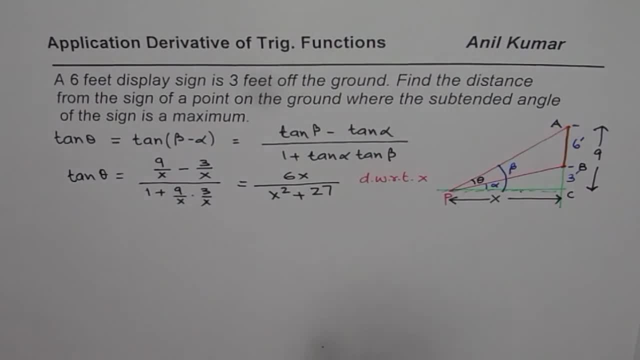 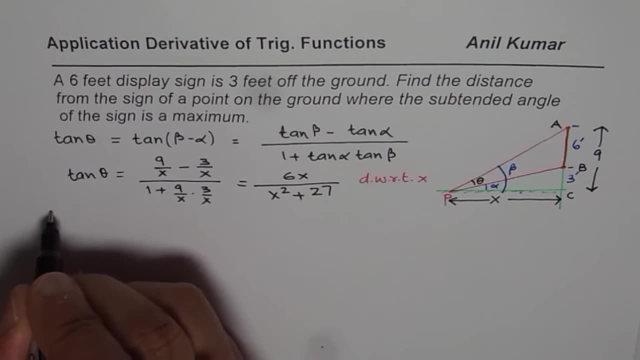 right on both the sides. So in that case, what do you get? So you get derivative of tan theta, secant squared theta. so we get secant squared theta times d theta. dx right Equals 2.. Here we'll apply the quotient rule. 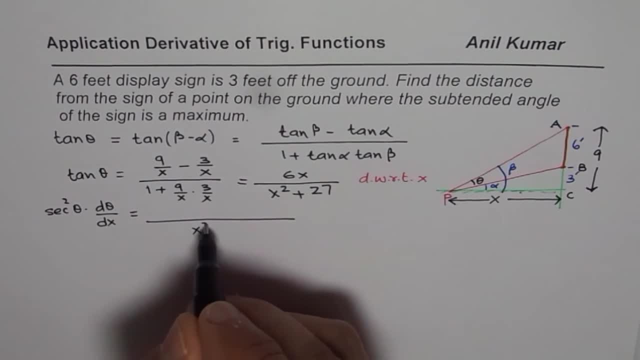 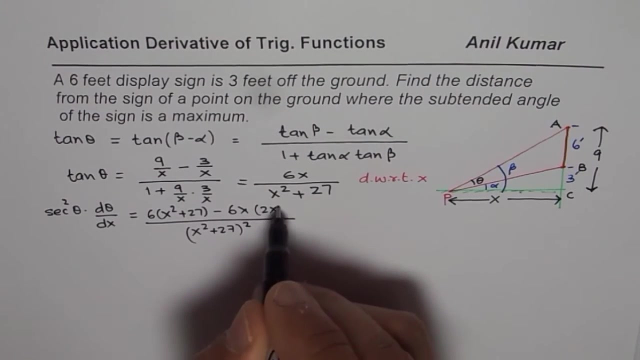 So we have, we have denominator as x squared plus 27. whole squared derivative of 6x is 6, 6 times x squared plus 27, minus 6x times derivative of denominator, which is 2x right. 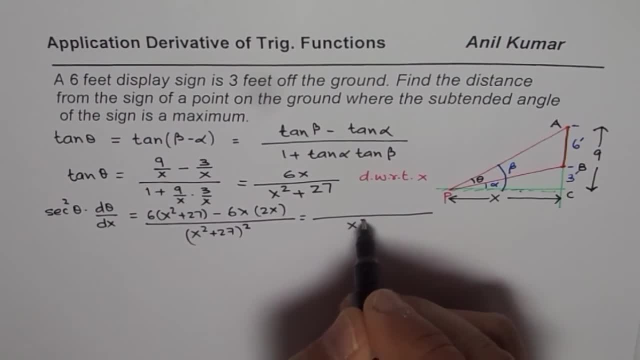 Now that could be simplified. We have x squared plus 27 whole squared and 6x squared plus 6 times 27,. I'm not multiplying them at present, and here we have minus 12x squared. So 6x squared minus 12x squared is how much. 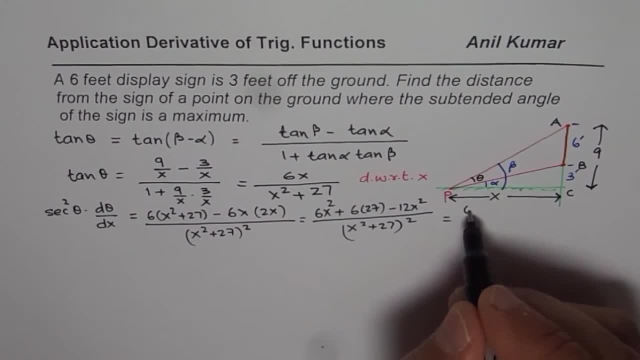 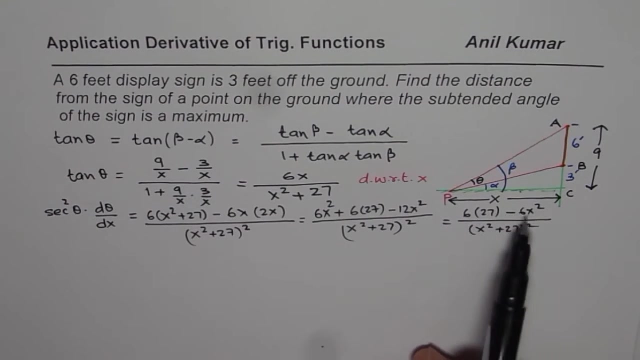 Let me continue here itself. It gives me 6 times 27 minus 6x squared in the numerator right, That is x squared plus 27 whole squared right. Here you can of course take 6 and 6 common, so we get 27 minus x squared, correct. 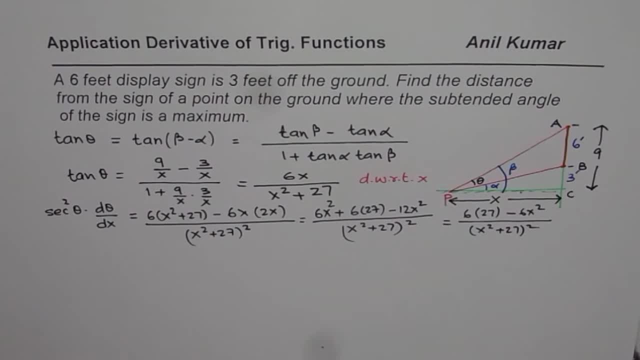 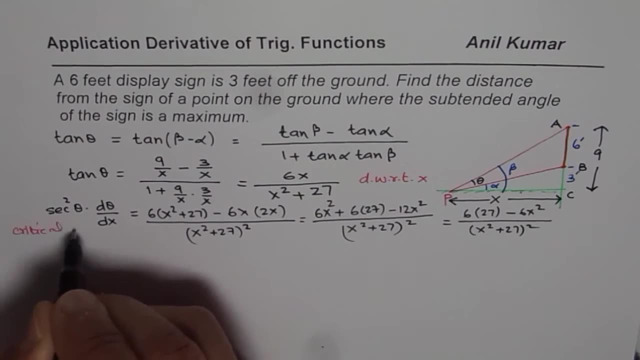 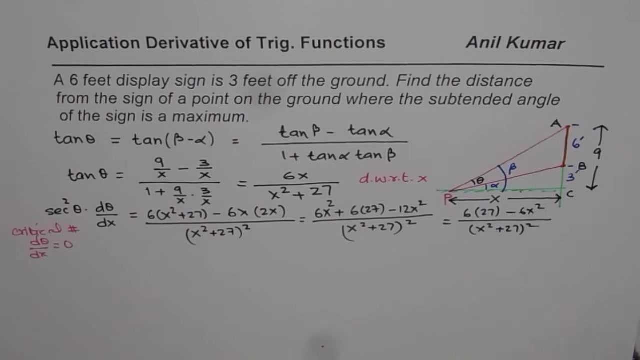 Now for critical number. for critical number, this should be 0, right. So for critical number d, theta dx equals to 0.. Now, that is going to be 0 only if we have this numerator as 0, right. That means we are saying 6 times 27,. 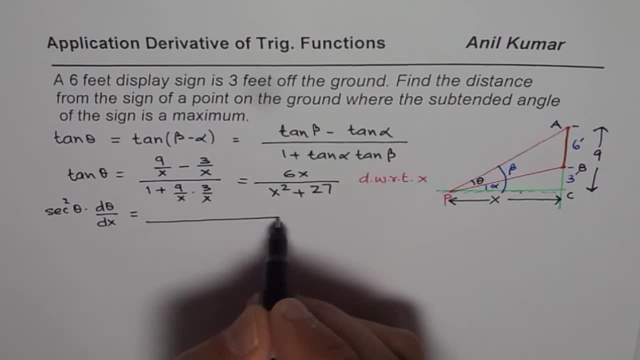 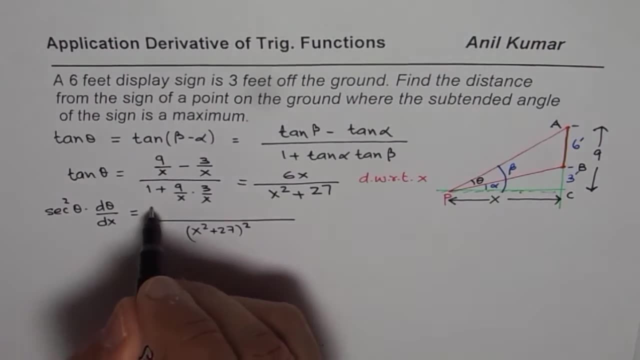 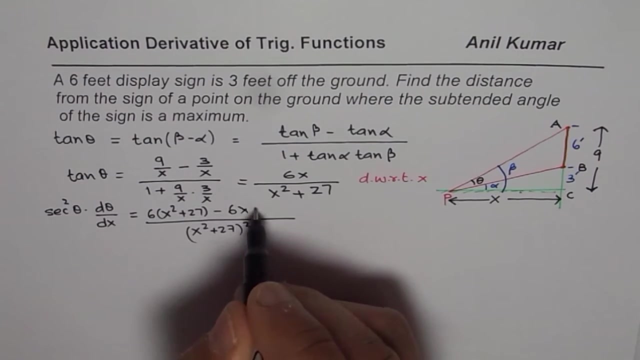 Here we'll apply the quotient rule. So we have: we have denominator as: x squared plus 27, whole squared Derivative of 6x is 6.. 6 times x squared plus 27 minus 6x times derivative of denominator. 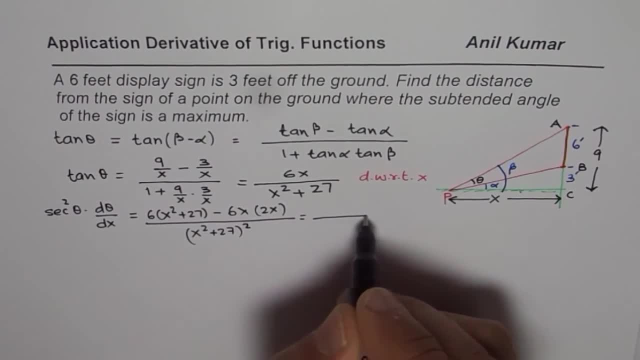 which is 2x. right Now that could be simplified. We have x squared plus 27 whole squared, And 6x squared plus 6 times 27 whole squared 6 times 27.. I'm not multiplying them at present. 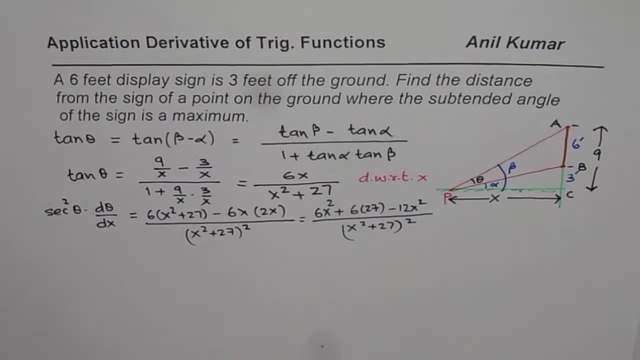 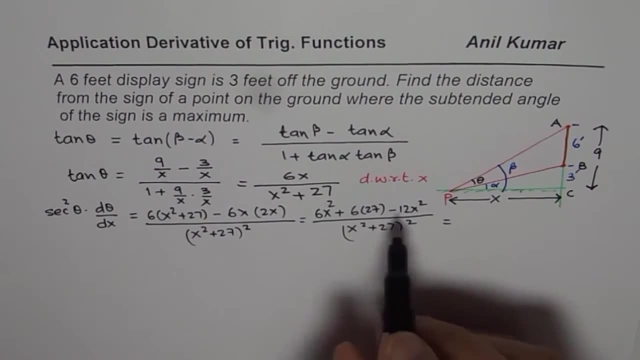 And here we have minus 12x squared. So 6x squared minus 12x squared is how much? Let me continue here itself. It gives me 6 times 27 minus 6x squared in the numerator right. That is x squared plus 27, whole squared right. 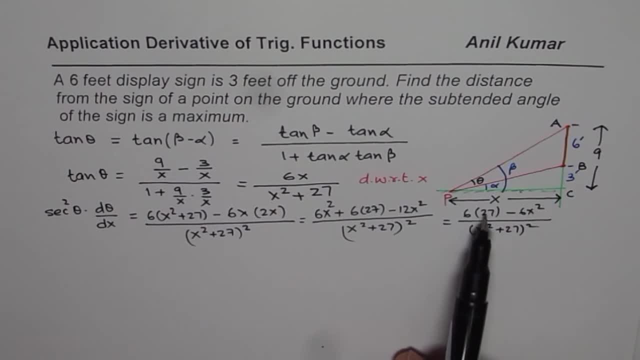 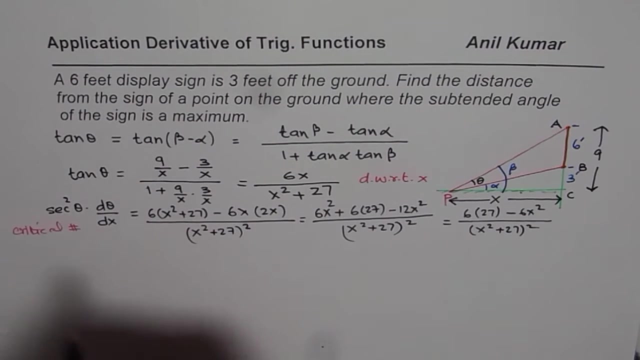 Here you can of course take 6 and 6 common, So we get 27 minus x squared, Correct. Now for critical number. for critical number, this should be 0, right. So for critical number d, theta dx equals to 0.. 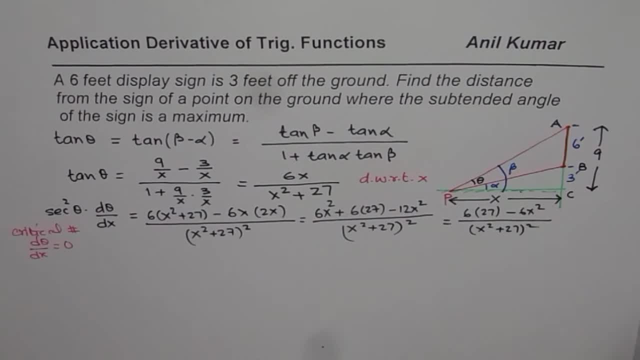 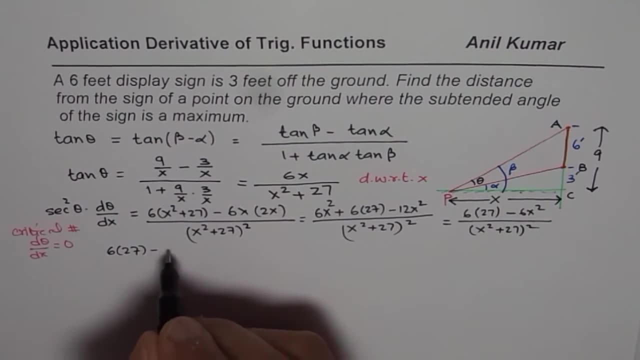 Now that is going to be 0 only if we have this numerator as 0, right. That means we are saying 6 times 27 minus 6x squared equals to 0, right. So we can now solve for x. So we get x squared equals to 6, and 6 cancel 27,, right. 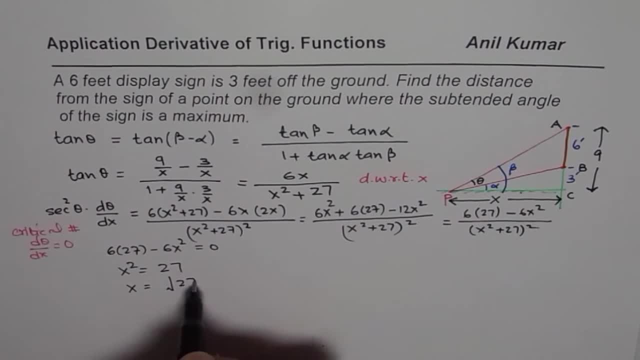 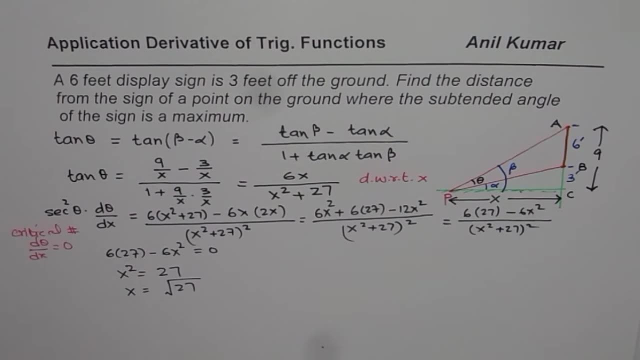 And x will be square root of 27.. Now, since x is the distance, we will take only the positive value. So that is our critical number, So we can approximate, So we can approximately find this number which is square root of 27.. 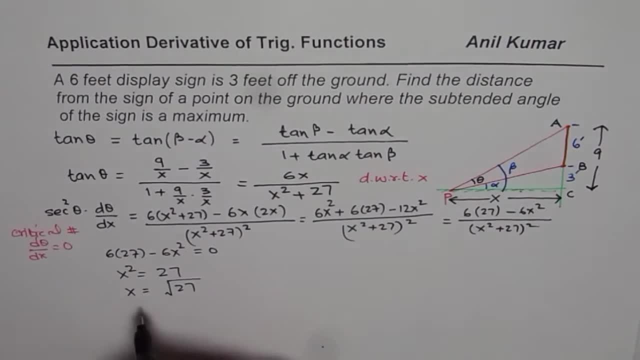 Yes, 3 square root, 3, 5.196, which is equal to 5.196.. Units will be in feet right, So that is the unit. Now the idea is to also show that this is indeed a maximum, So this is very important to show. 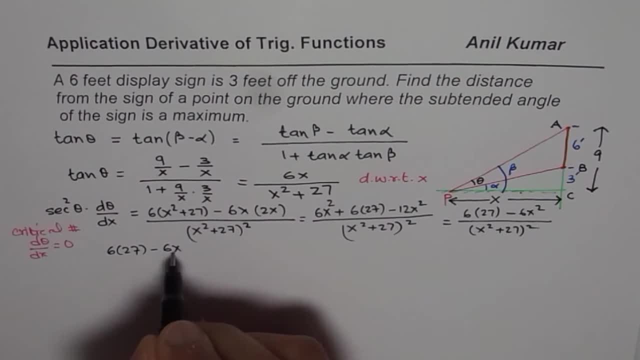 minus 6x squared equals to 0, right. So we can now solve for x. so we get x squared equals to 6 and 6. cancel 27,- right, And x will be square root of 27.. Now, since x is the distance, 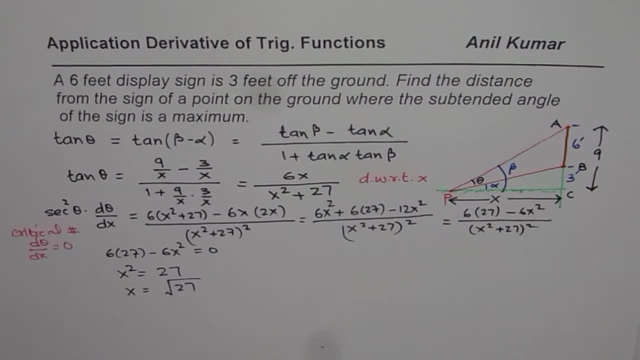 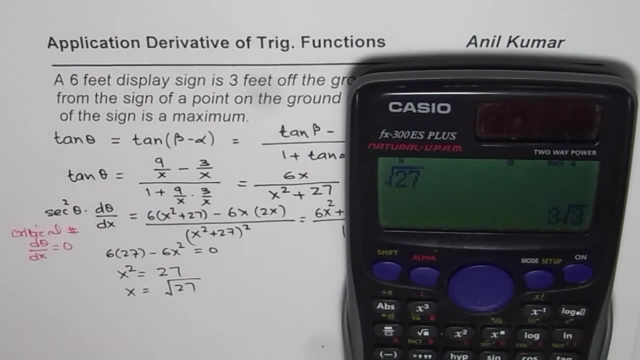 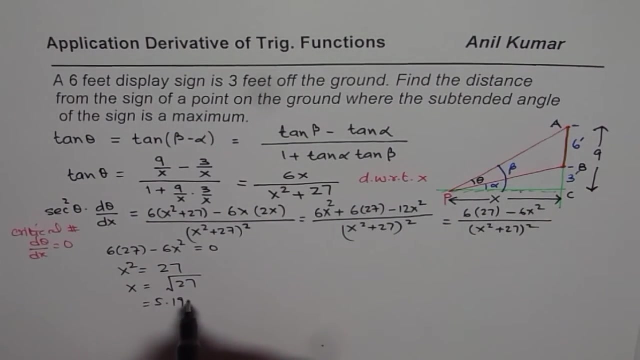 we will take only the positive value. So that is our critical number. So we can approximately find this number, which is square root of 27.. Yes, 3, square root 3, 5.196, which is equal to 5.196, okay. 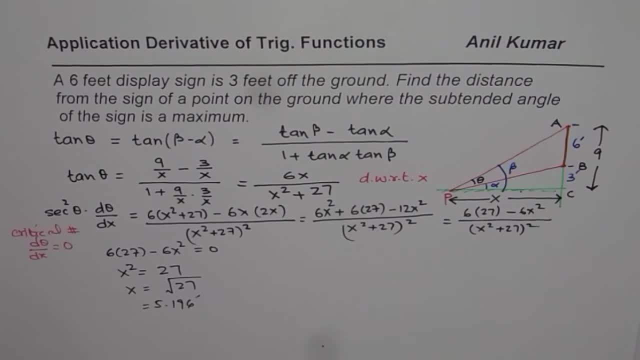 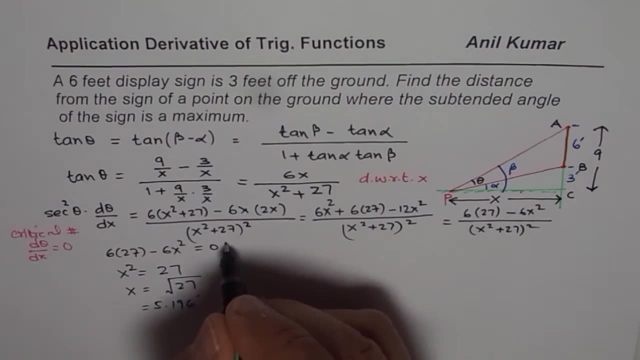 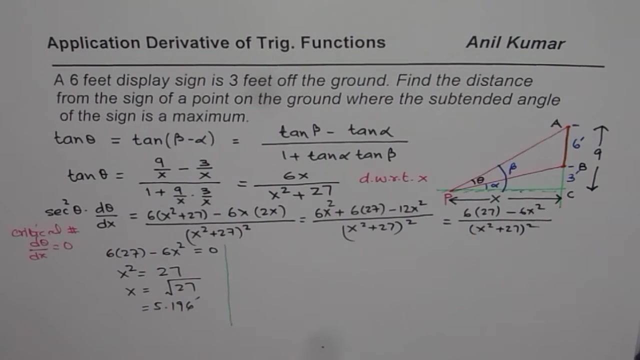 Units will be in feet right. So that is the unit. Now the idea is to also show that this is indeed a maximum, So this is very important to show. Now for that, we will analyze d theta dx. So we will analyze d theta dx. 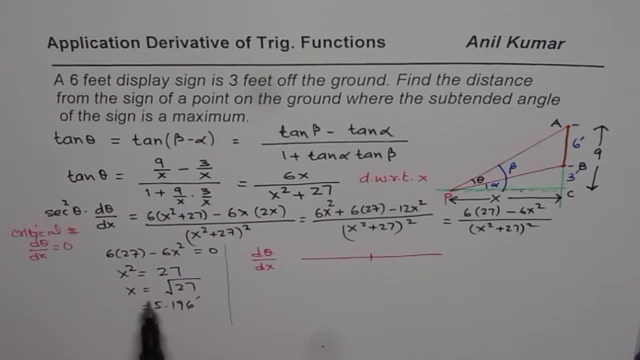 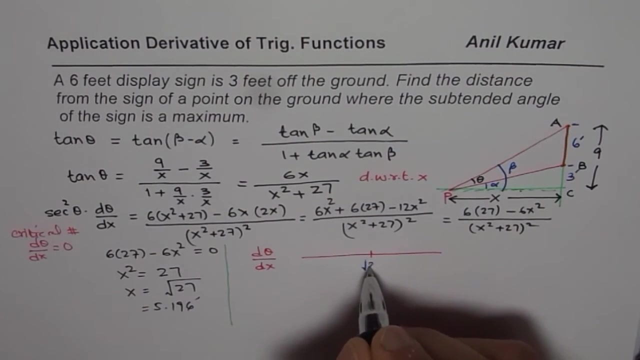 on points which are either side of square root of 27,. right So, square root of 27, and see what is correct. So we can write square root of 27 here, which is a right here if I am taking a bigger number. 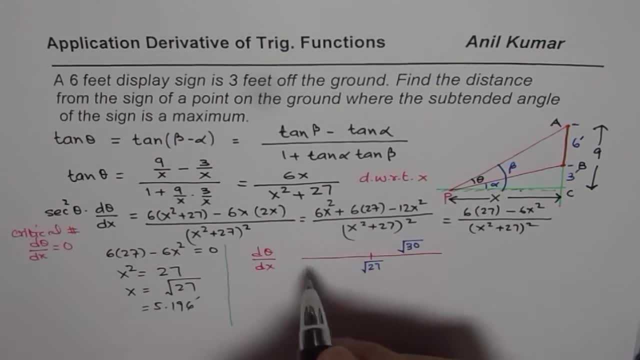 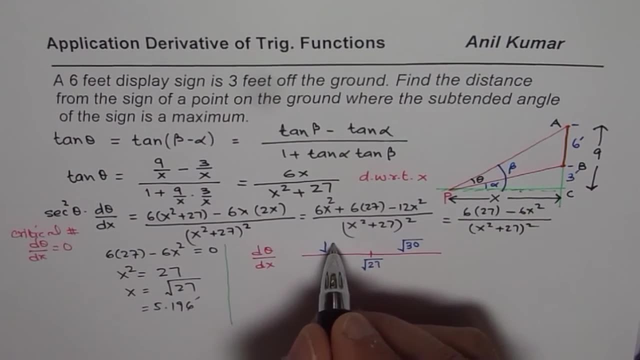 let me write square root of 30,, which is a bigger number, and square root of, let us say, 25 is 5, anyway, Because it is x square. let me write square root of 26,. okay, it doesn't matter, okay. 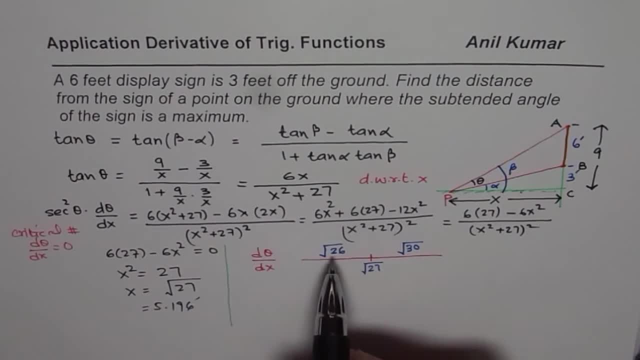 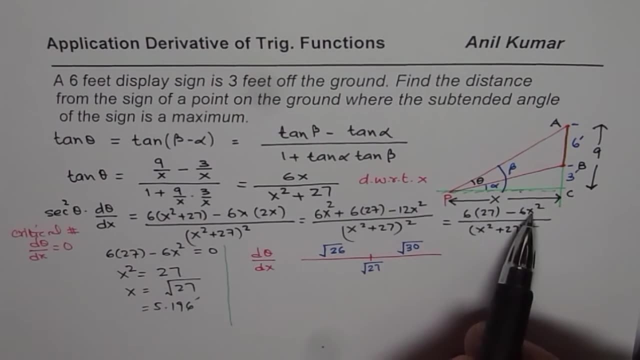 I didn't want to write square root 25.. Now, if I substitute denominator is positive, correct. If I substitute here 26 square, it is 6 times 27,. this is 6 times 26,. of course that is going to be a positive value, right. 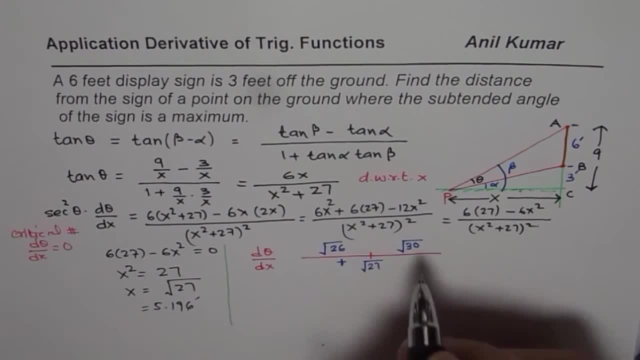 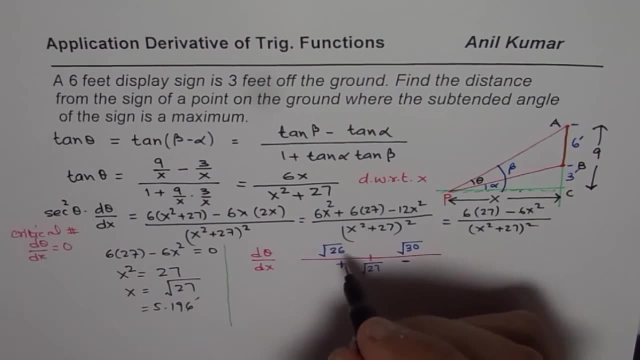 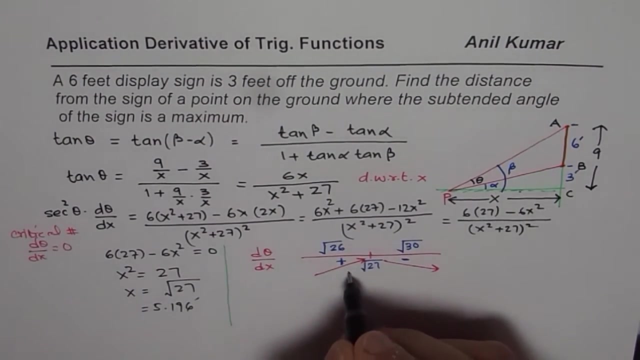 So this is going to be positive, right? If I substitute 30, then this minus sign will be here. it will be negative. So clearly, on the left side, derivative is increasing and then it is decreasing and that indicates a maximum right. 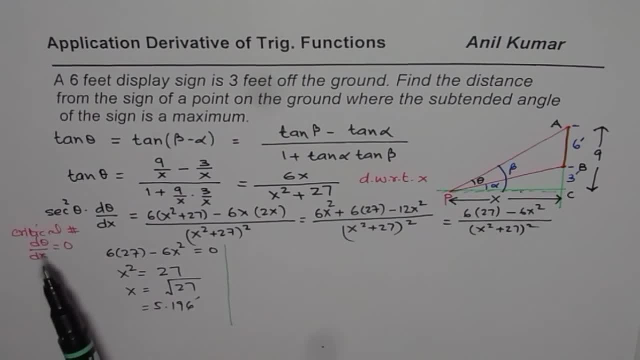 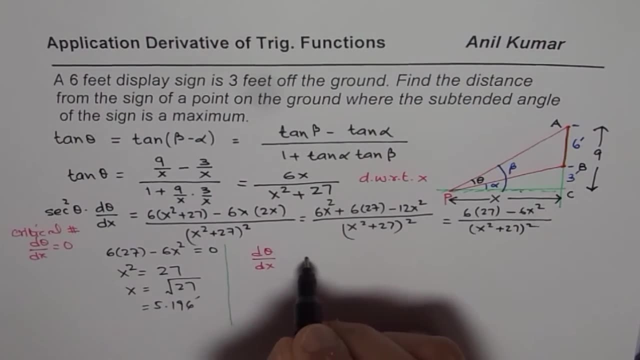 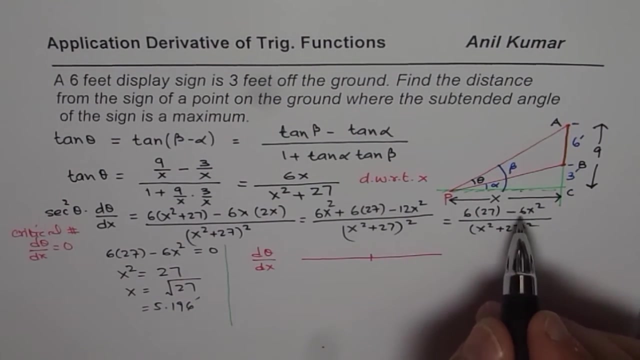 Now for that, we will analyze d theta dx. So we will analyze d theta dx on points which are either side of square root of 27,. right, So, square root of 27, and see what is correct. So we can write square root of 27 here, which is a right. 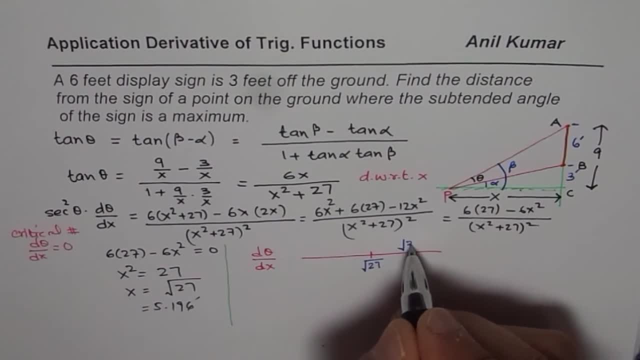 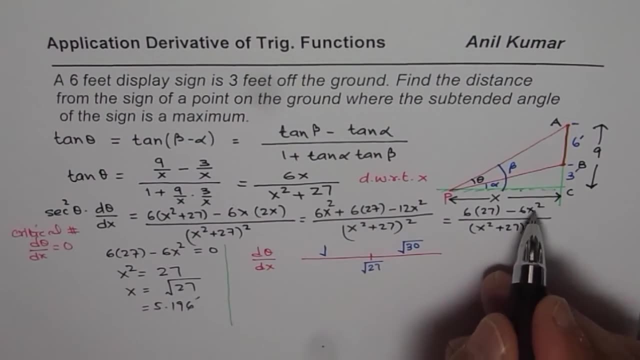 Here, if I am taking a bigger number, Let me write square root of 30, which is a bigger number, And square root of, let us say, 25 is 5. anyway, Because it is x square, let me write square root of 26.. 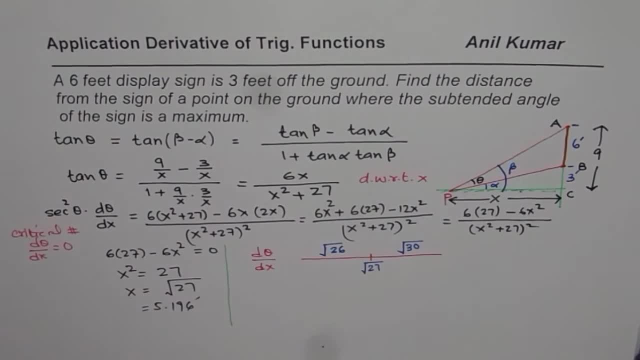 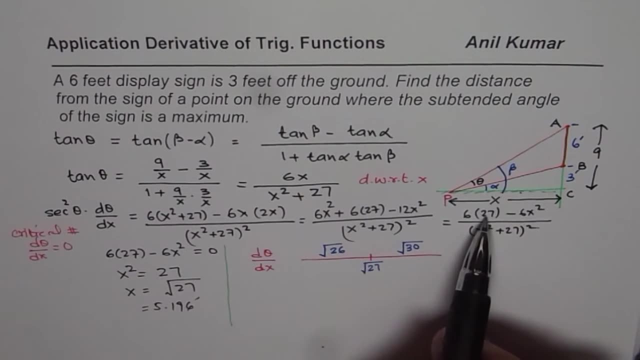 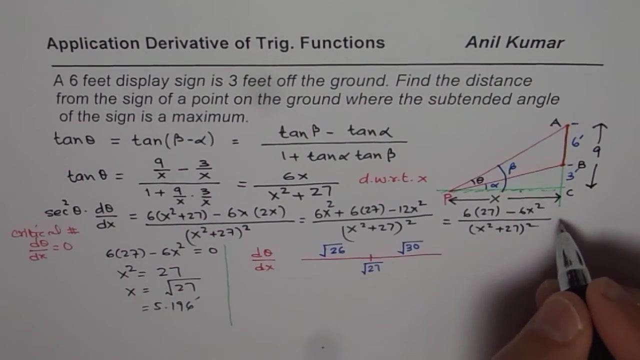 Okay, it doesn't matter. Okay, I didn't want to write square root 25.. Now, if I substitute denominator is positive, correct. If I substitute here 26 square, it is 6 times 27.. This is 6 times 26,, of course. 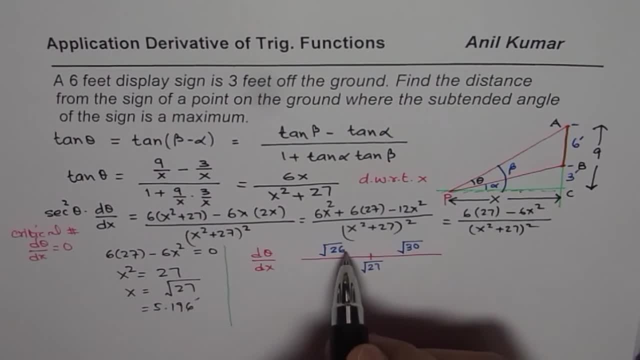 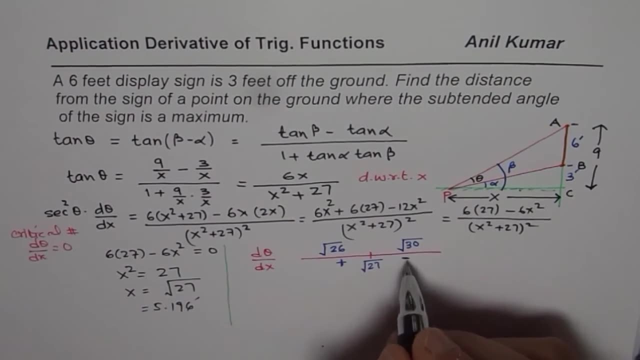 That is going to be a positive value, right? So this is going to be positive, right? If I substitute 30, then this minus sign will be here, it will be negative. So clearly, on the left side, derivative is increasing and then it is decreasing. 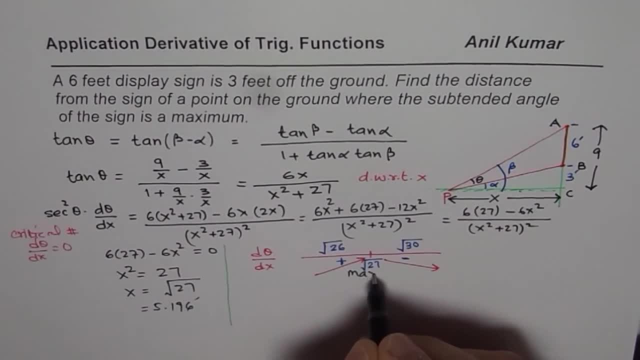 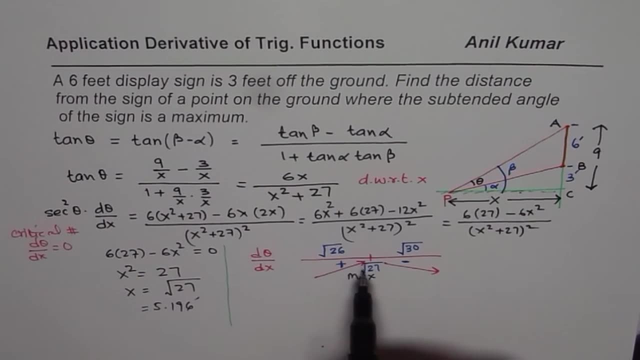 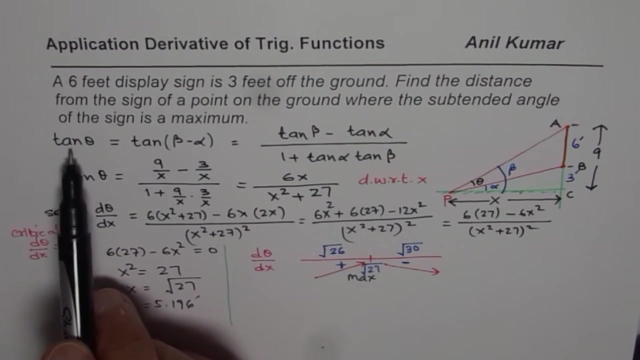 And that indicates a maximum right. So we have a maximum for square root of 27,, correct? So for x value of square root of 27, we do get a maximum, correct? That is very clear. Now let's get back to the angle itself. 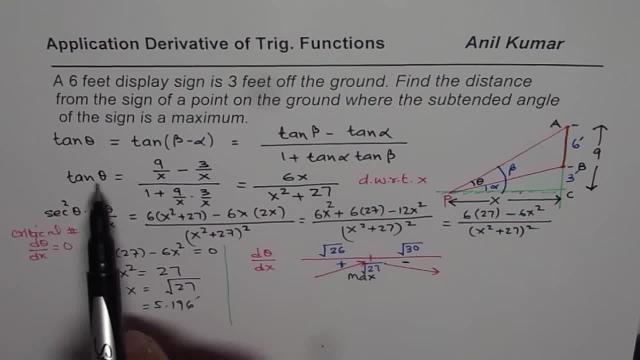 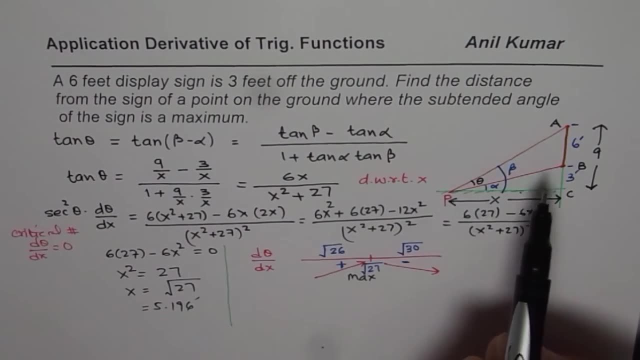 We started with tan. theta equals to all this. So what is theta? We have to still find that right. So what is theta Distance? we know How far away. So say, find the distance from the sign of the point on this, where the substantive angle is. 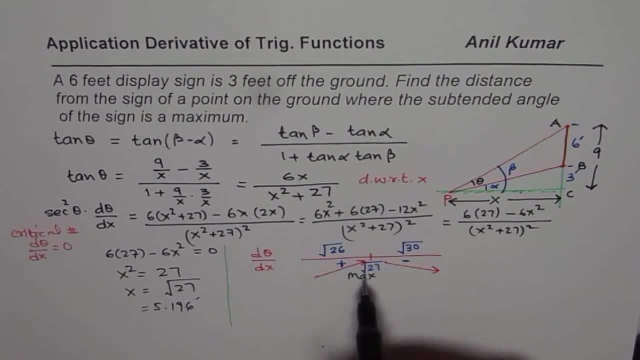 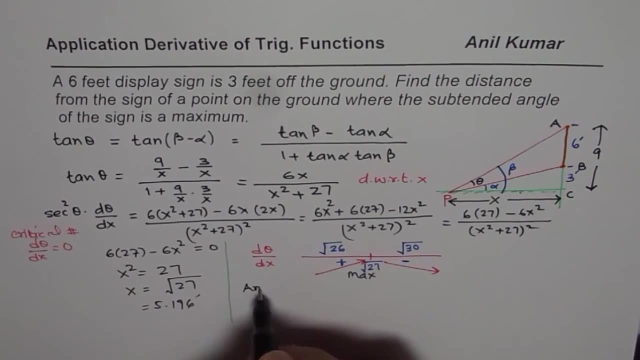 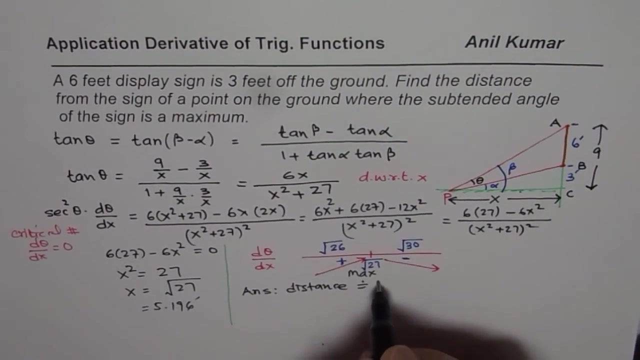 Okay Now. so in this particular example, we need to find the distance correct. So the distance is correct. So we get our answer. And the answer is: distance should be approximately 5 point. let us say 2 feet, right? 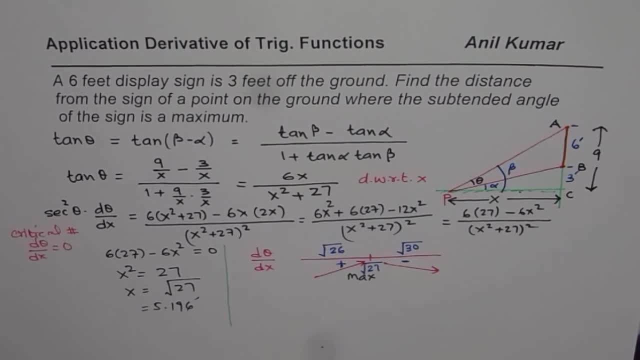 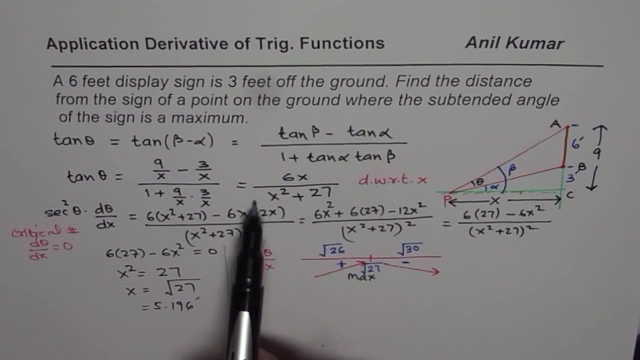 So we have a maximum for square root of 27,, correct? So for x value of square root of 27, we do get a maximum, correct? That is very clear. Now let's get back to the angle itself. We started with tan. theta equals to all this. 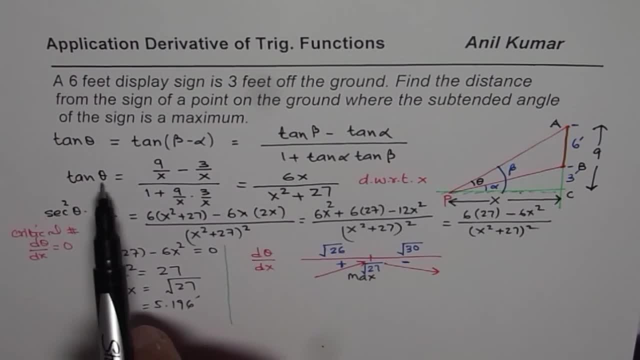 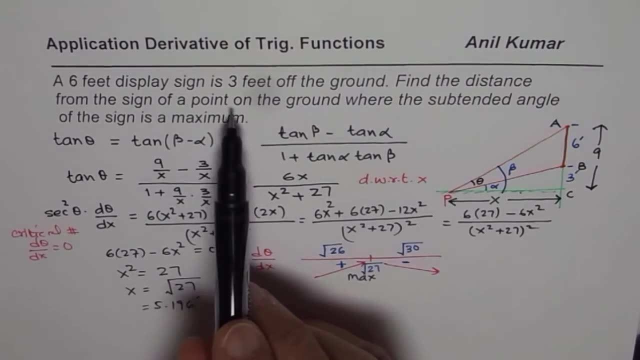 So what is theta? We have to still find that right. So what is theta Distance? we know How far away. So say, find the distance from the sign of the book. point on this where the substantive angle is Okay. 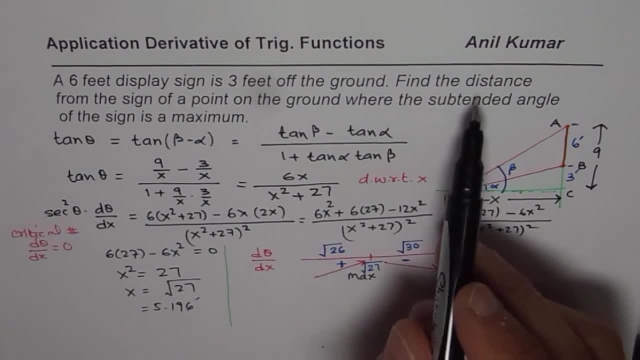 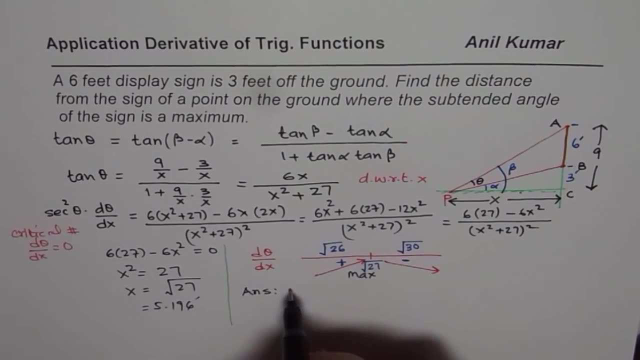 Now. so in this particular example, we need to find the distance correct. So the distance is correct. So we get our answer and the answer is: distance should be approximately 5 point. let us say 2 feet, right? 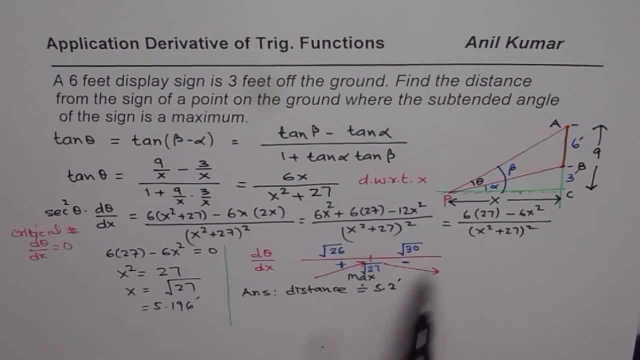 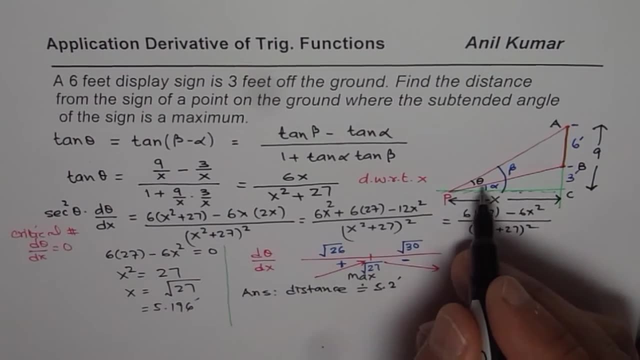 5.196, right, 5.2 feet, So that is the distance. At times you may be asked for the angle right, So at times you may be asked for the angle. So the question for you is: 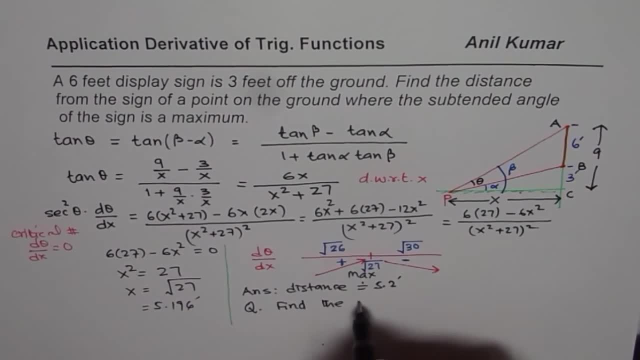 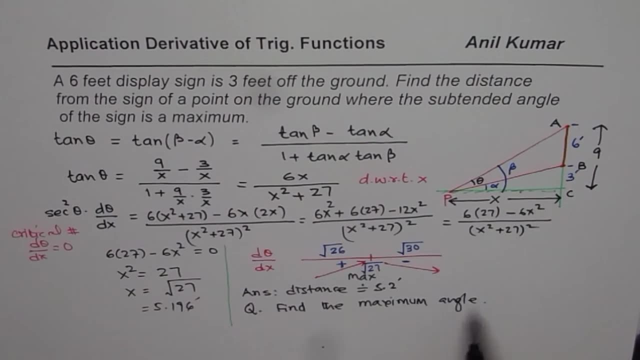 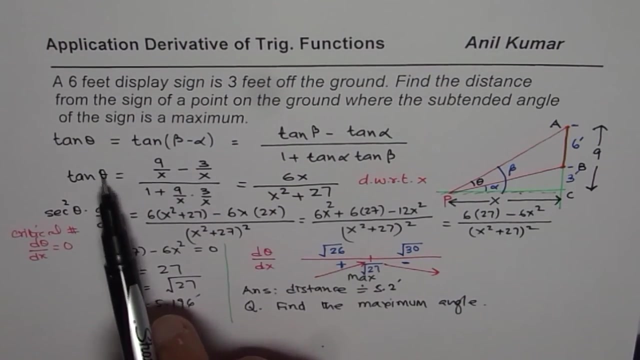 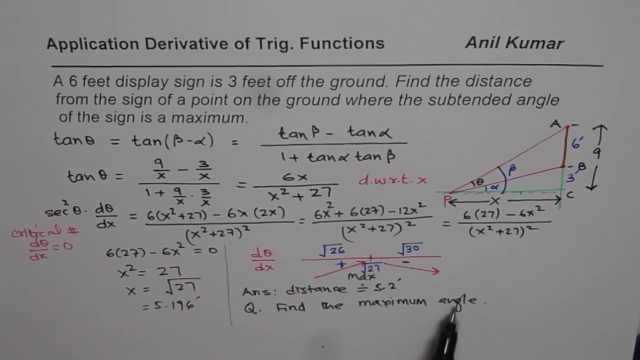 find the maximum angle. Now, to find the maximum angle, you need to substitute this value of square root 27. in this formula, 10 theta equals to 6x over x squared plus 27, and then 10 inverse will give you the angle theta right. 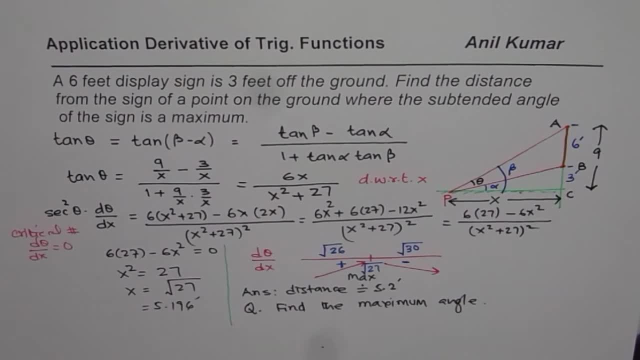 So that is how you can actually find the maximum angle. also, I hope in this example you understand how to solve such questions right. It is very interesting and important example. You will get many questions like this. You could get a question like: 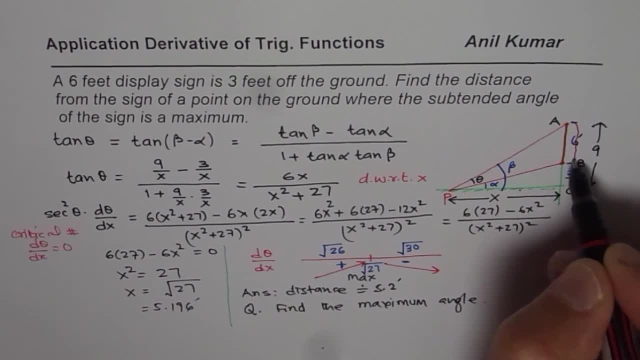 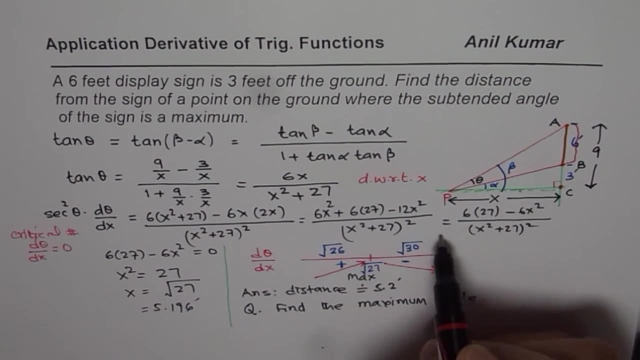 imagine this is kind of a hockey net right And a player is 3 feet away. and if it moves outside perpendicular to this way, what could be the distance from the goal line so that you get the maximum angle? So like that also. 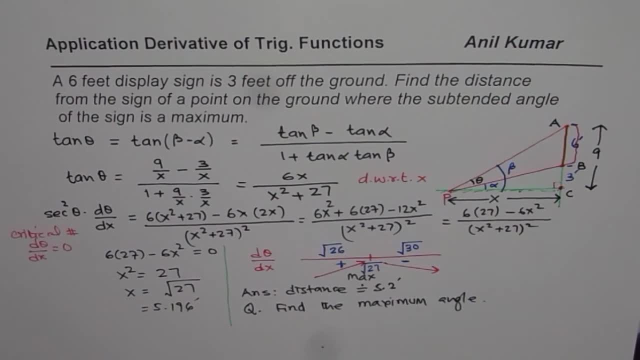 we could have a question correct, And this type of approach which you have taken as difference of angle is seen in many examples. So I like you to go through this example, properly understand the concept, how we have used difference of angle.